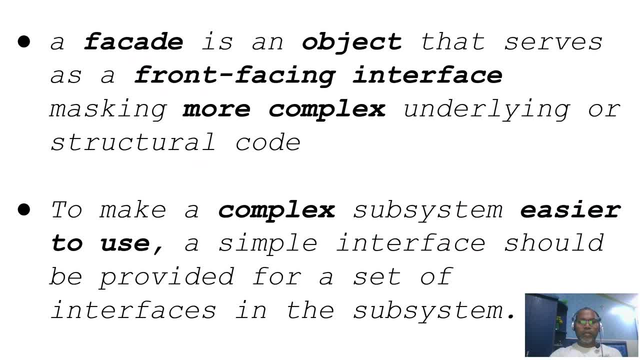 So, as per the definition, Fasad is an object. Fasad is an object that serve as a front facing interface for a client And masking all more complex underlying structural code What they mean. That means we have a system For accessing those system. you have to access module 1, module 2, module 3, module 4.. 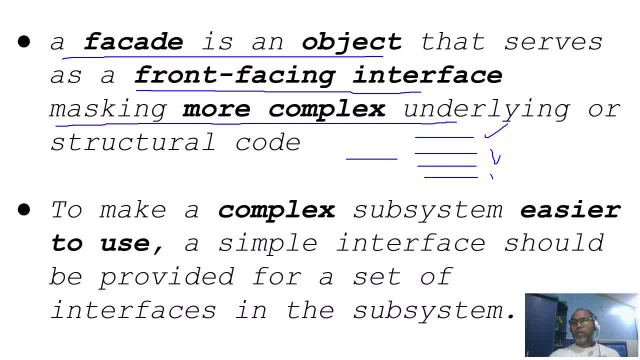 And finally, after that, your system is working. This is a kind of a complex system, So whenever anyone want to access, they have to do step 1 and step 2.. Maybe we have to invoke API 1, API 2,, API 3 and final come, your product is done. 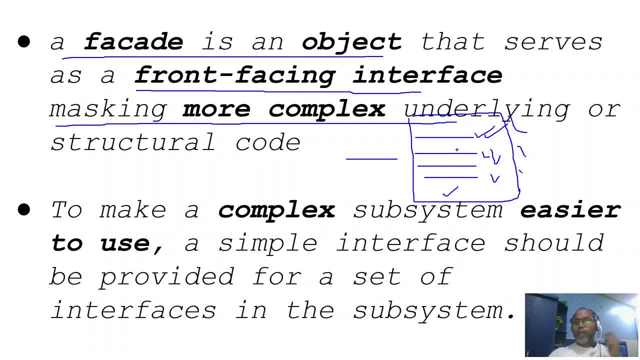 So instead of multiple API call, multiple setup statement performs. That can be made simple. Simple That Fasad say We write a simple client facing object, Just client know the minimum changes. So to Fasad, just make the complex subsystem easier to use Simple. 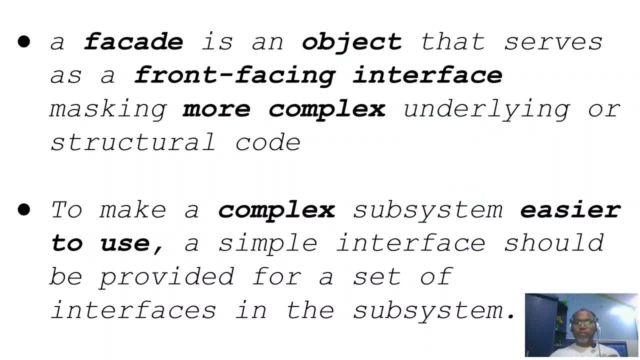 Okay, Fasad design pattern, say To make a complex subsystem easier to use, Okay. So whatever your system designing, that's okay. But we have also taken care we have to offer simplest way. Any can use my code, any can use my product, any one can use my system. 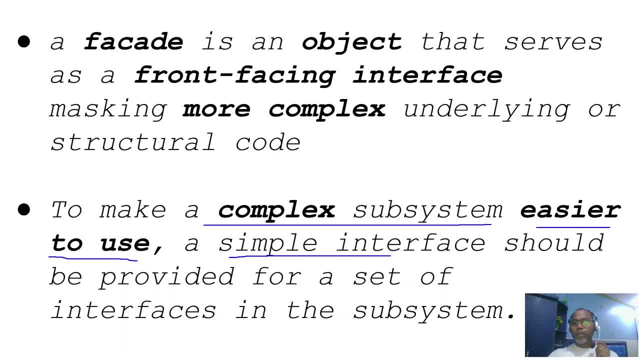 So just give a simple interface that should provide for the client, So that the client can easily interact with your lots of subsystems, with your lots of subsystem, whatever the your system have. so in short, this pattern help us. he seek just to find one kind of client facing object. okay, 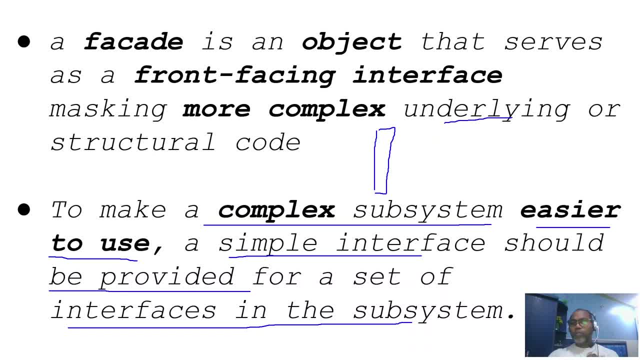 underling, underling. whatever your system doing, whatever a system doing, perform a set ofestess. maybe you are doing. lets then set up box. you will do. maybe you had enough. you remote call may be, I don't know if in database call. so why these set up steps? client should know and might be client don't know in which. 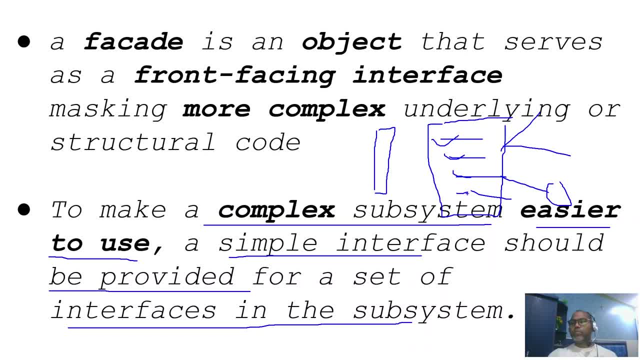 order, you have to invoke the set of steps. so instead of exposing this complex system to the client, we say, hey, client, we are offering you one. faintly, are just you this my simplest interface and you can pass what required input and I am giving you the only response. rest of internal happening: lots of API call, database call. 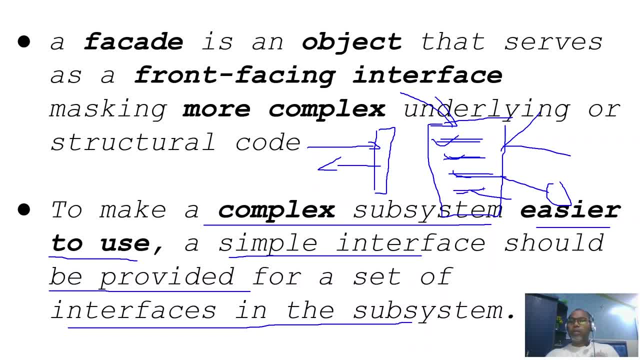 system processing, all are done internally. so that is the way facade say, facade is just. they are not getting any business logic, they are not doing anything. just say you whatever as a software provider you are providing, just in so that you are giving a simplified interface for the end grain, whatever the 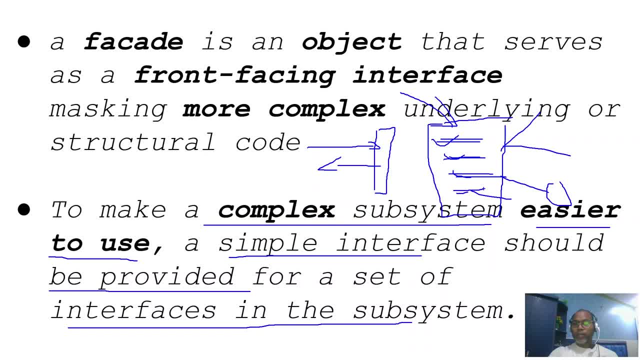 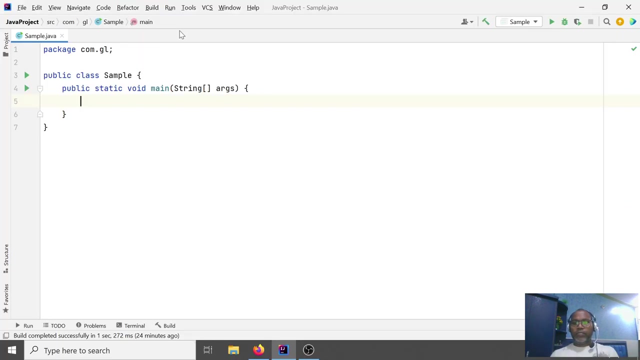 person you are going to use. your system code may be any, any system may be can use your system code or any human being. so you have to, just you have to just write one simplified version. that is the facade. so let us look the example and then say you how it's easier to use means, what the facade means. so let us 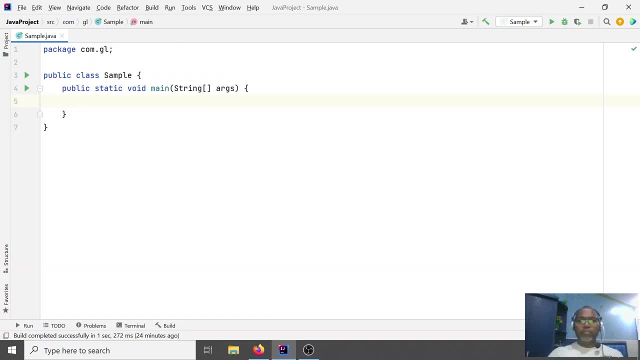 example, here based, let's say, scenario: you, what we are, can do. let's you are going to buy some product, let's you want to buy maybe any product, any product you want to buy. so for this subsystem, for this subsystem, lots of entity work, maybe there is one product. 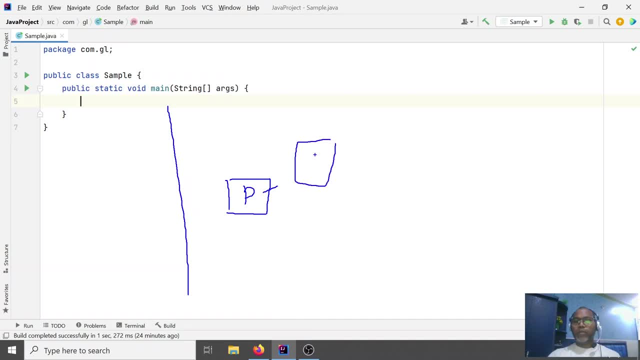 for this product just belong to the particular company. might be this product you want to. some maybe buy product kind of thing. which product? list of product which maybe you are buying product. maybe you need some kind of a payment. someone want to buy it. they have some payment. so these some set of entity internally work to complete your buying a. 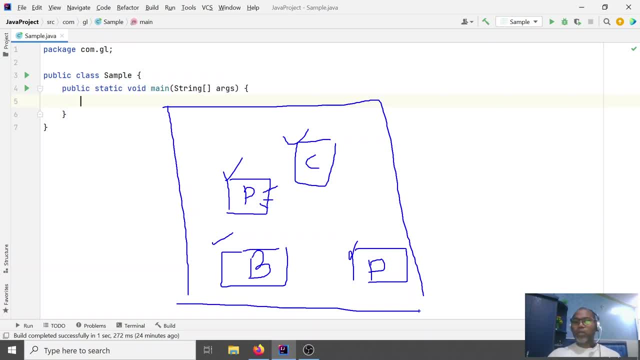 particular product. okay, so you can define independent component and you have to ensure that there are some set of steps you have to perform to buy a particular product. so let it's like this: First buy product concept and then think how we can write simplified version for 추천. 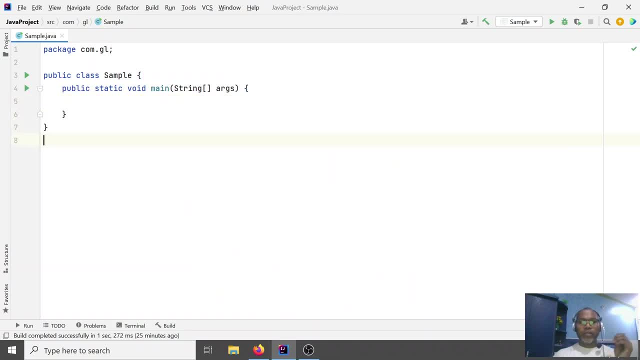 ok, so, as the monologue is going to use, we have a class like we final product, with a product class and keywords class. yes, please, Akil, string product name: okay, and this product must be belong to for company. let's see the company class. company have a. let's name name okay, and just let's. 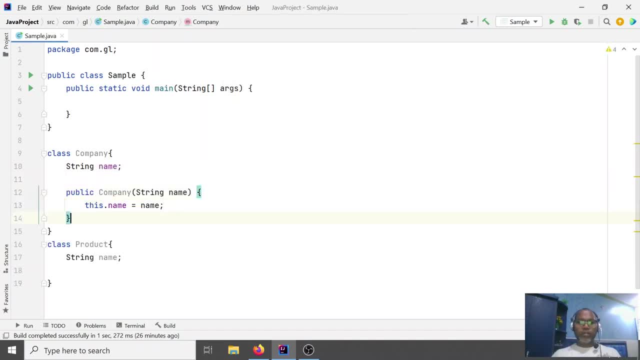 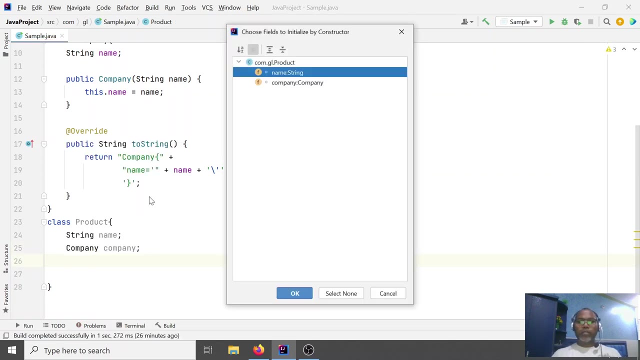 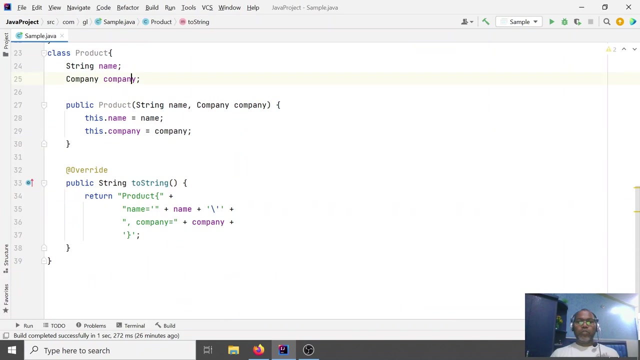 see insert. okay. and now your come. now you have a, your company name. okay, now just in slide with the constructor and just suffer your twisting method, okay. so now we have a product on. let's see someone want to buy the product. of which product they are buying? 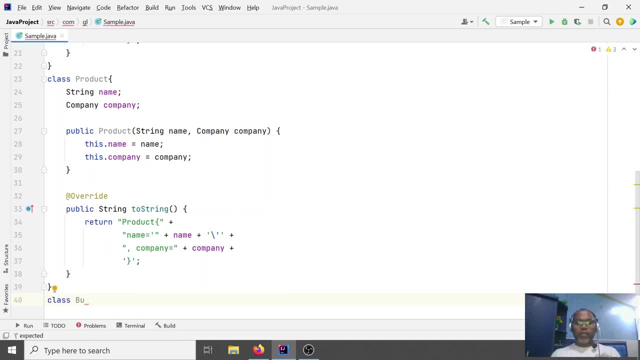 let's we have a class man, key by product. let's keep buying product, have a which product you are buying. okay, let's key, just seen inside you the constructor and just write a twisting method. okay, now, if someone buying a perp must have a kind of a class which they receive payment. 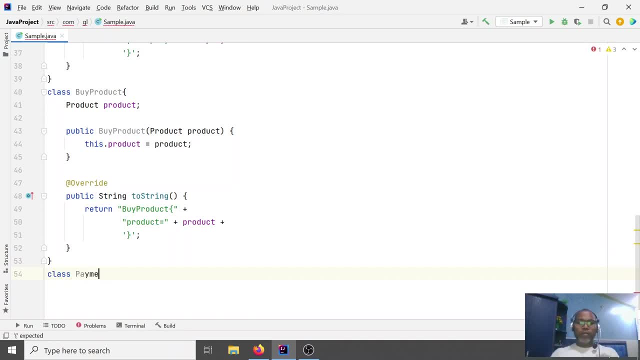 okay now, if someone buying a perp must have a kind of a class which they receive payment. okay now, if someone buying a perp must have a kind of a class which they receive payment, payment, payment, and for which buying product you are receiving a payment. let's 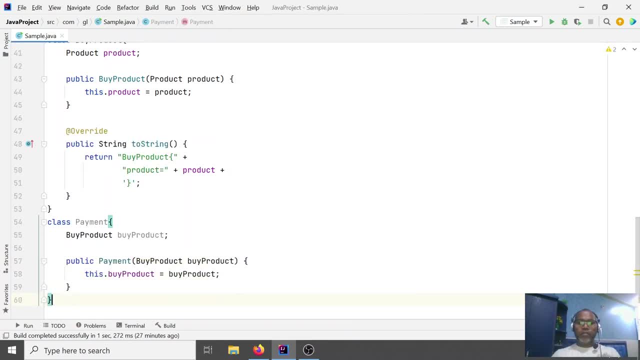 payment payment and for which buying product you are receiving a payment. let's: payment payment and for which buying product you are receiving a payment. let's: in style, you the constructor, and just in style, you the constructor. and just in style, you the constructor. and just over a twisting method, this is just for. 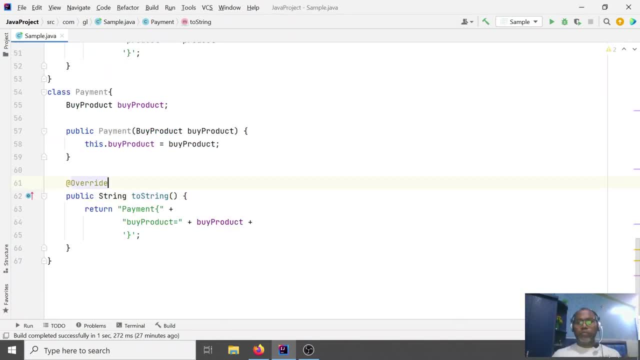 over a twisting method. this is just for over a twisting method. this is just for demo. I am NOT going to more detail, but demo. I am NOT going to more detail, but demo. I am NOT going to more detail, but this is simple twisting method. now this. this is simple twisting method. now this. 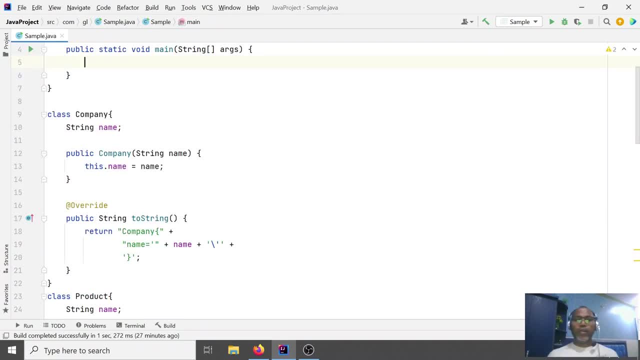 this is simple twisting method. now, this is our subsystem in this way you are is our subsystem in this way you are. is our subsystem in this way you are offering this, someone can buy my product. offering this, someone can buy my product. offering this, someone can buy my product. so let's key, I am going to buy pro, so 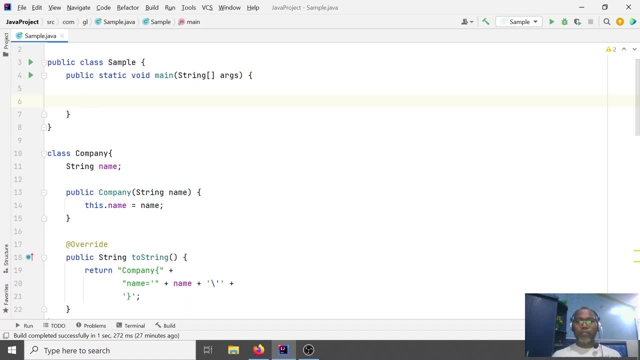 so let's key, I am going to buy pro. so so let's key, I am going to buy pro. so whenever I am selecting product after, whenever I am selecting product after, whenever I am selecting product after that, I have to save pay something so that I have to save pay something. so 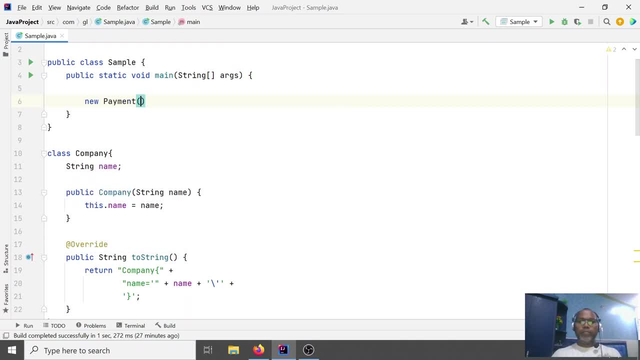 that I have to save pay something. so let's say I'm going to pay payment. okay. let's say I'm going to pay payment. okay. let's say I'm going to pay payment. okay. do you know for payment we have to? do you know for payment we have to? 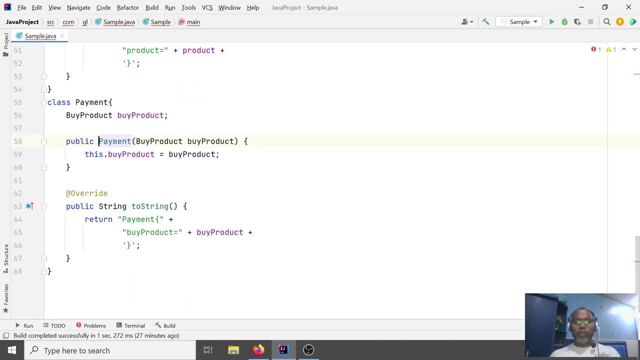 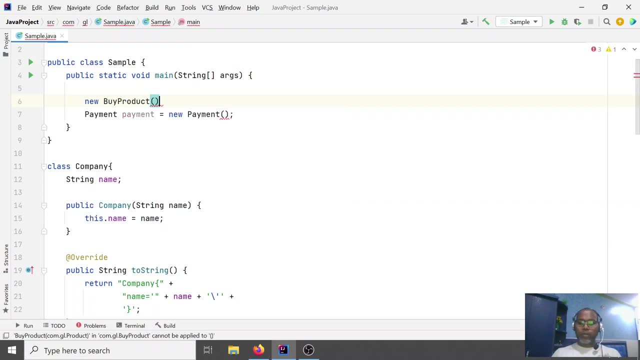 do you know for payment we have to which payment? asking which product we which payment, asking which product we which payment, asking which product we have by. so we have to create like a new have by. so we have to create like a new have by. so we have to create like a new buying product. which product I am going? 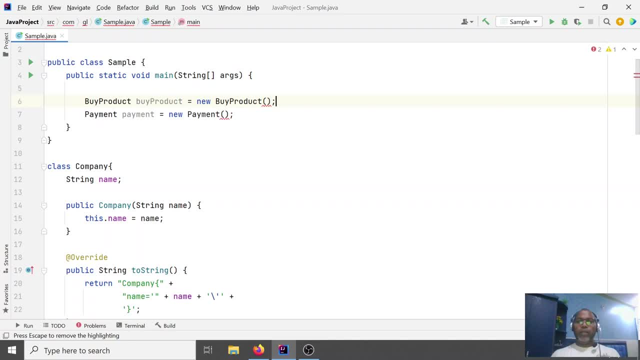 buying product, which product I am going buying product, which product I am going to buy. so buying products? say, tell me to buy. so buying products? say, tell me to buy. so buying products, say tell me, though, which product you are buying. so though, which product you are buying. so 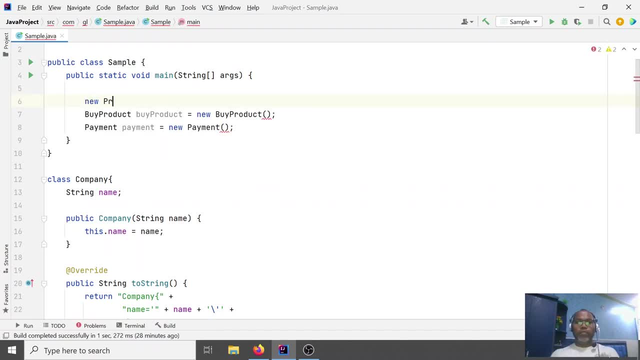 though which product you are buying. so might we have to create a buying. might we have to create a buying, might we have to create a buying product first. you may be product, now say product first. you may be product, now say product first. you may be product, now say product, want which product. let's see I. 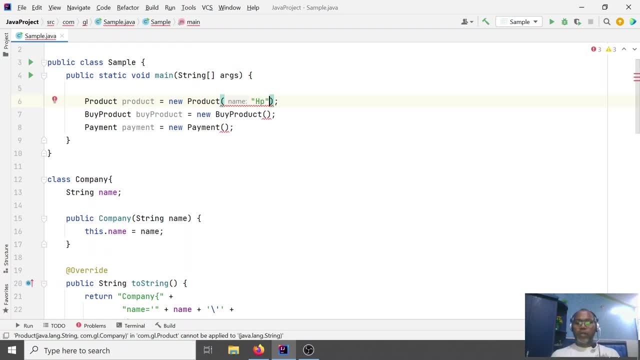 product want which product. let's see I product want which product. let's see I want a SP product and from which company want a SP product and from which company want a SP product and from which company might be when the credit company object might be when the credit company object. 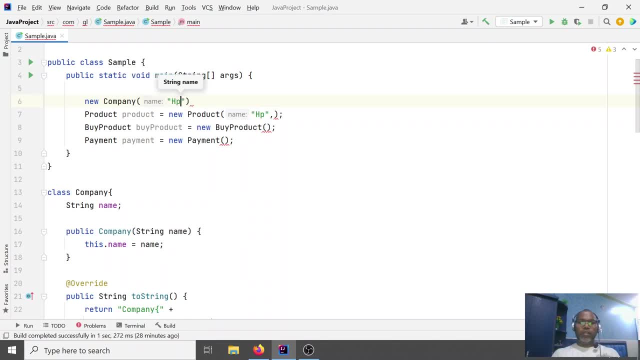 might be when the credit company, object: company, let's see SP company. and here, company, let's see SP company, and here, company, let's see SP company. and here you pass, here it's be I, here you pass you pass, here it's be I, here you pass. 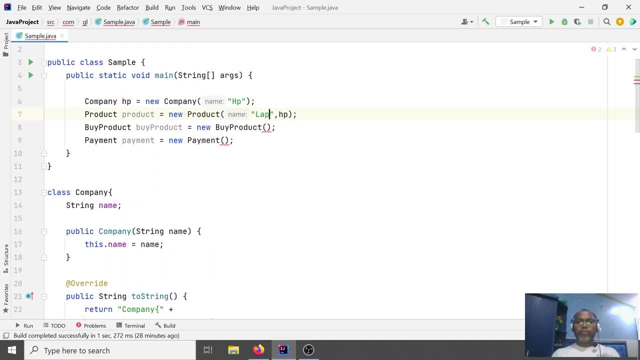 you pass, here it's be I. here you pass which product my product may be left off. which product my product may be left off. which product my product may be left off. now here, say: I'm this product I am. now here, say I'm this product, I am. 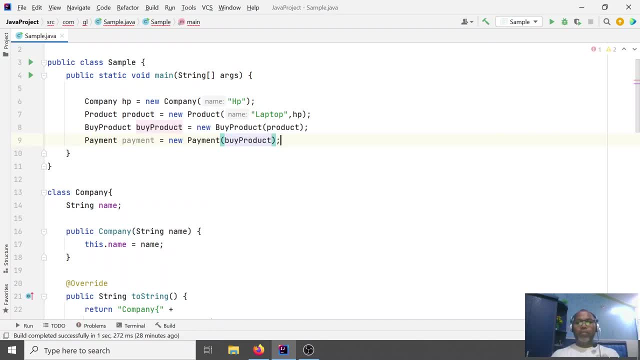 now here say I'm this product I am buying and this is the my buying buying and this is the my buying buying and this is the my buying product, and after that you can say just product, and after that you can say just product, and after that you can say just let's keep him and define kind of one. 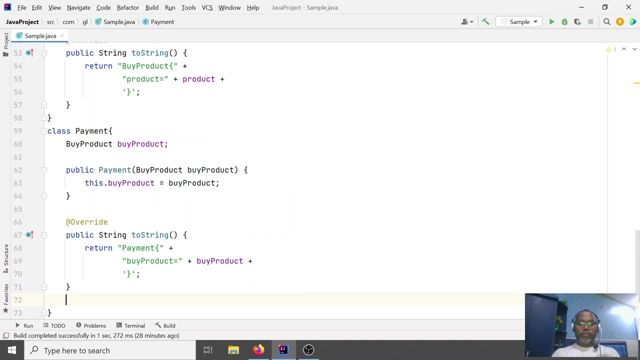 let's keep him and define kind of one. let's keep him and define kind of one of my turn, like of my turn, like of my turn, like bye this, this, this payment, payment, payment, payment, payment, done, done, done, I'm gonna just feet, I'm gonna just feet. 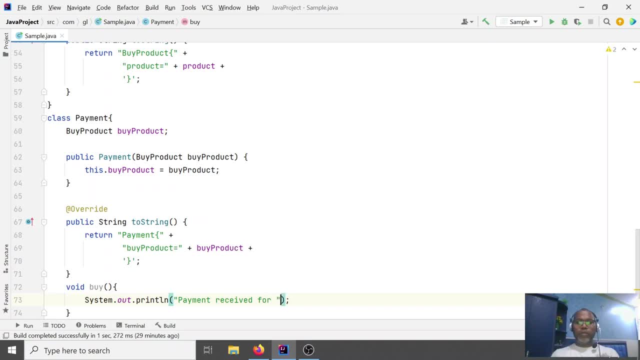 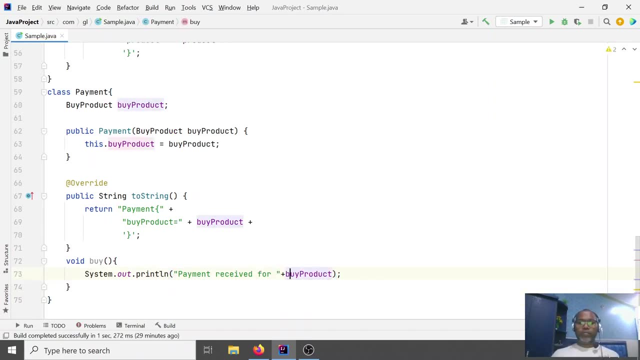 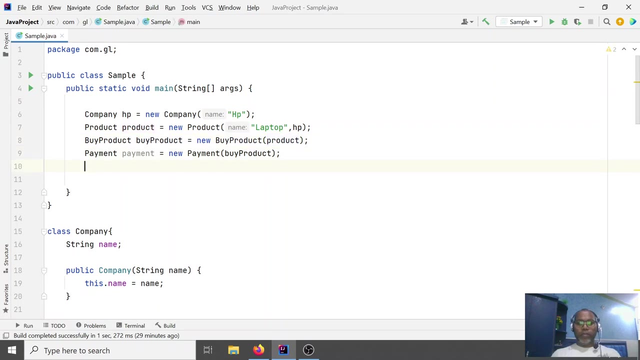 I'm gonna just feet: what product which, what product, which product? Let's key: buy product Done. So now this is the system, and now you say paymentbuy. So now your system is working properly. Anyone, any client, want to access your subsystem. they have to follow these setup steps. Payment received for buying product. 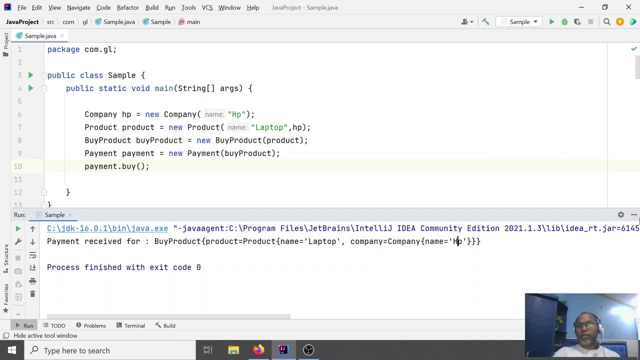 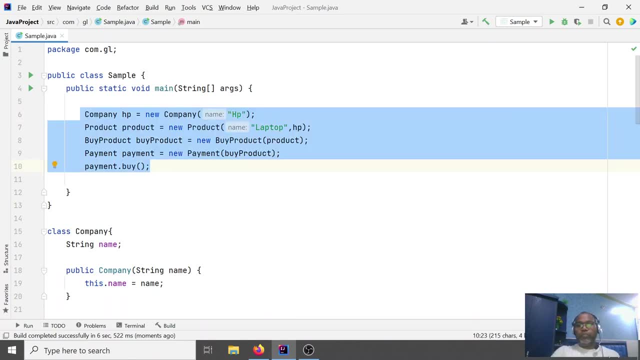 this product name, this laptop and company this. But this is the kind of a we as a developer know key for creating a payment object. we need a first buying object. After that we need again product object. Product need the company object. This is the kind of very complex Client don't know about the internal how. 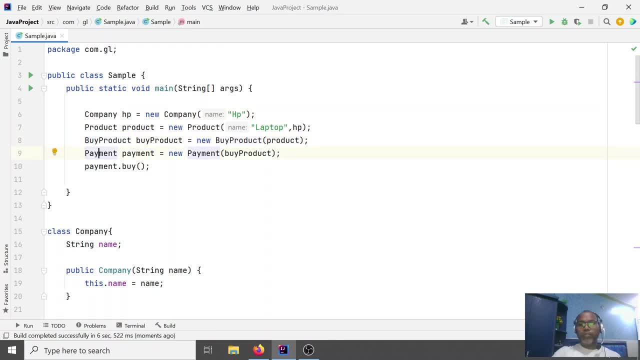 you are buying product, what the payment is. So this is worked, Your system is worked, It is working properly. But this is not more easier for client. If someone want to use your code, they have to write this setup steps. This is kind of complex steps, So why not? 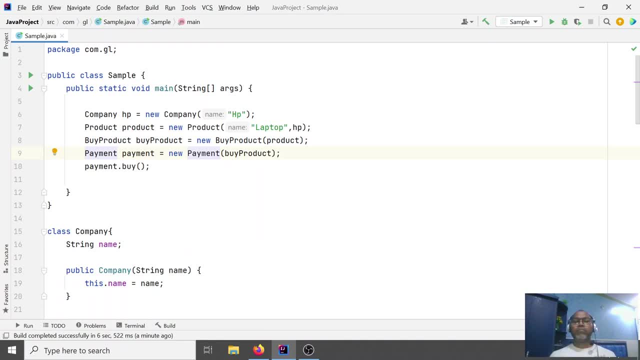 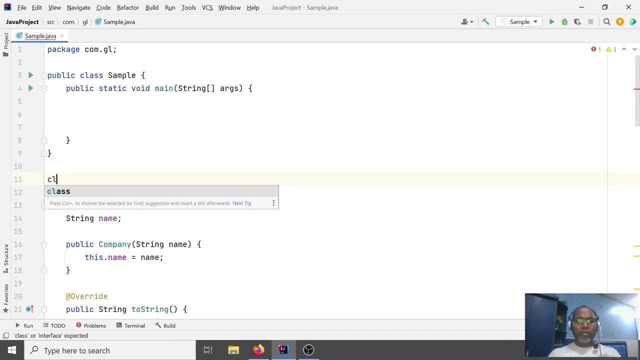 we offer some kind of simplified version All day. So this is facade, say, whatever your complexity to access your system, Can we just come find in one object and just say you can use my simplified version. So instead of this, just here and write like one class. 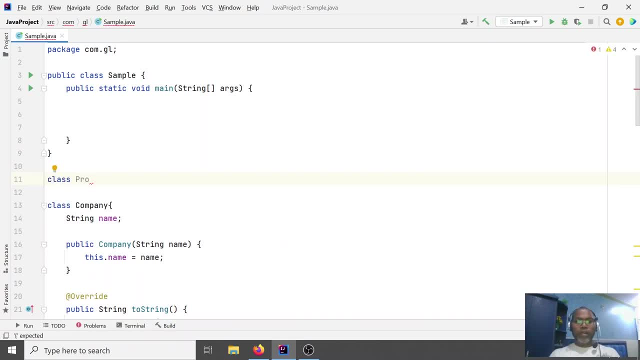 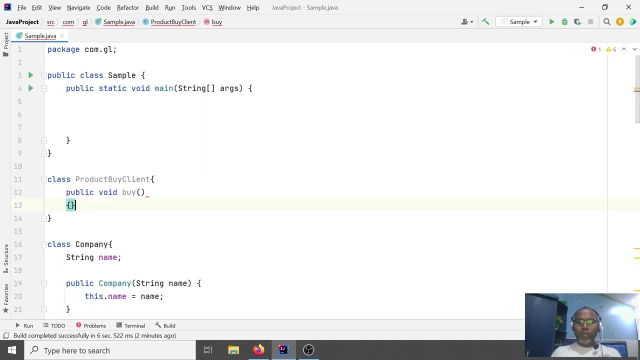 is what we are going to do. This is what we are going to do, Okay, And whatever the complex things you have just to insert. So here what you need: you need a company name. just take your input, string your name, and here you just place the company name, whatever the 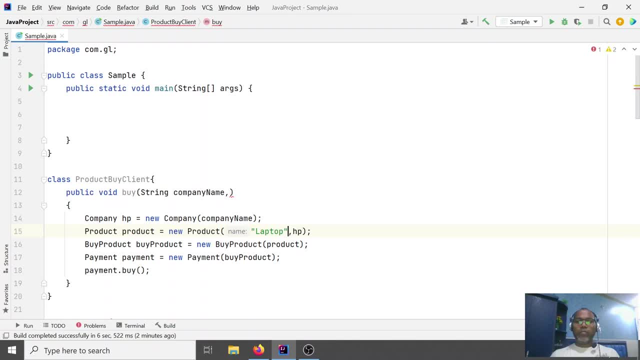 company name you want And here the product you want. So there should be string like product name. just replace with ok. now you have accomplished. now just say client. this is my client facing interface. someone want to buy my product. just use my buy product. 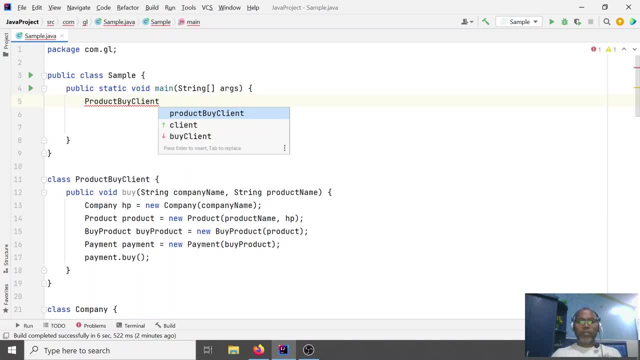 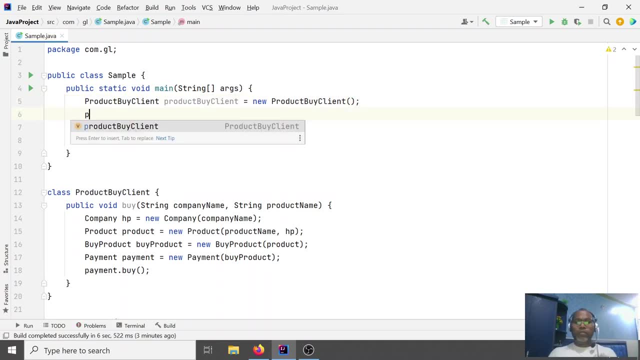 client just buy product. client equal to just client- just create the object and simply say I am going to buy the product. he say: just give me the company name. just I want to give a del and what is the product I want to? laptop, just done. 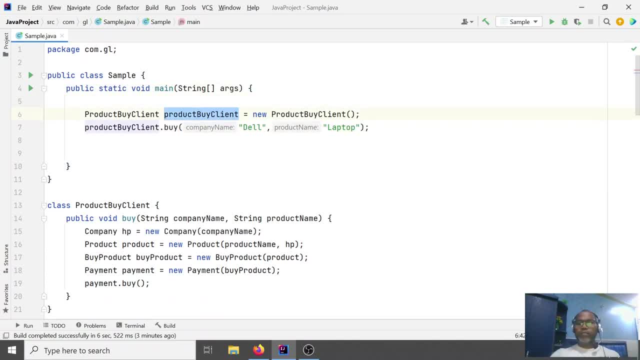 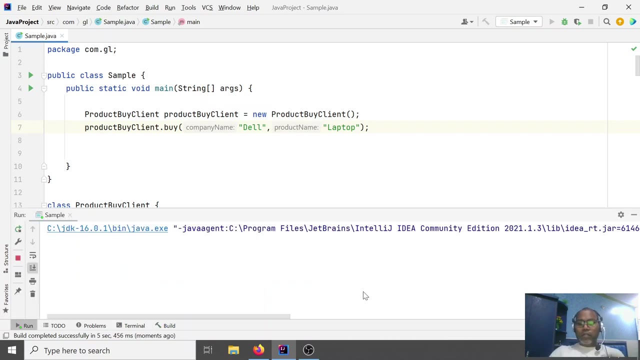 So client here only have one object- this is kind of facade- just say buy, this is my company name, this is my product, I want just run it. So all the hurdle, the procedure, the steps, now the same pay matrices for it and client. 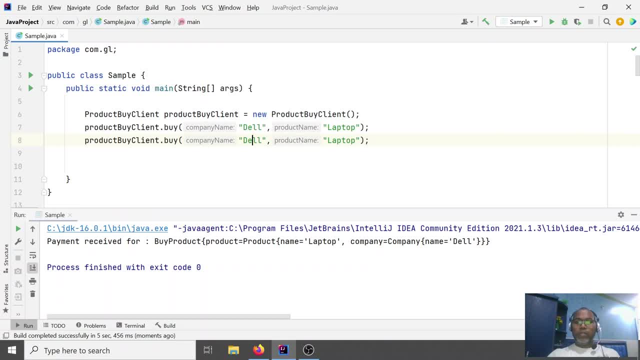 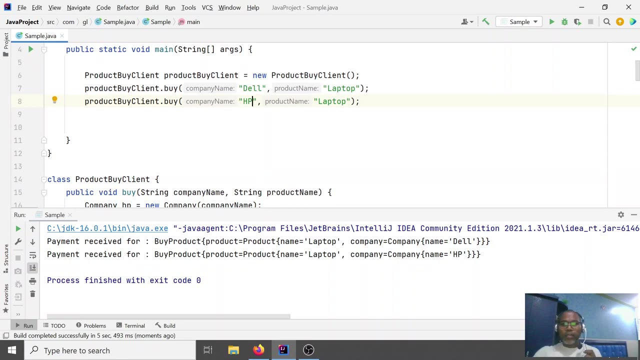 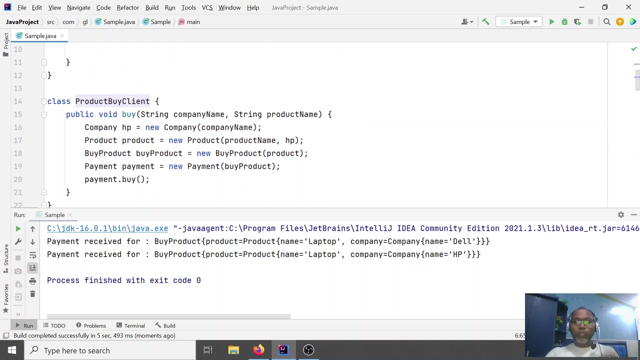 can buy any another product. So simply let us say they want HP laptop. they can easily buy right. So here this client means, whatever your sub system is, Design, you know how the system can anyone use. If someone don't know internal about you might be cannot access your system, or they. 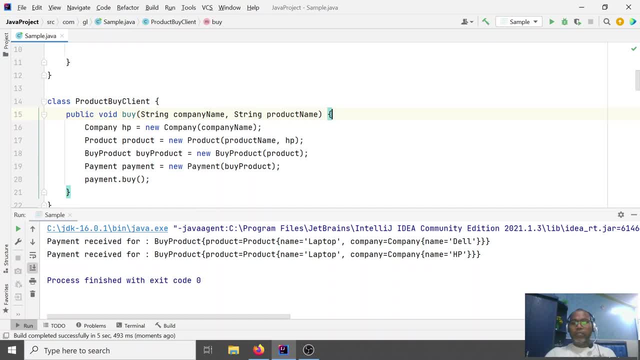 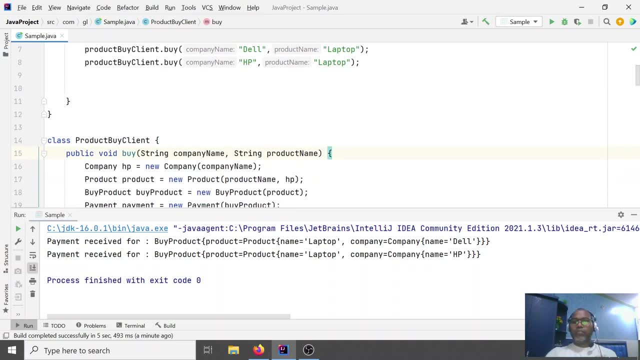 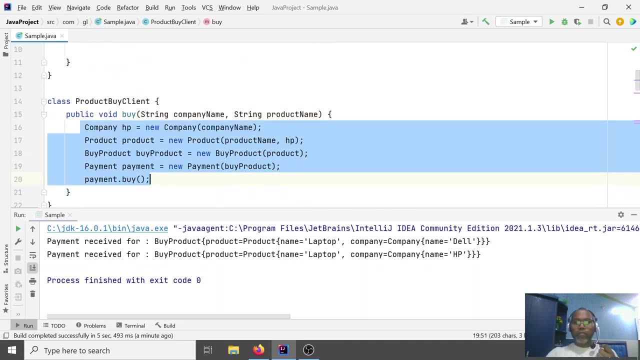 facing problem. So you, as a product owner, you know the system well. you just write the one simplified version So anyone can want to access, be access. So whatever the complex flow you have, Ok, Just write a simplified version. this is like for client. 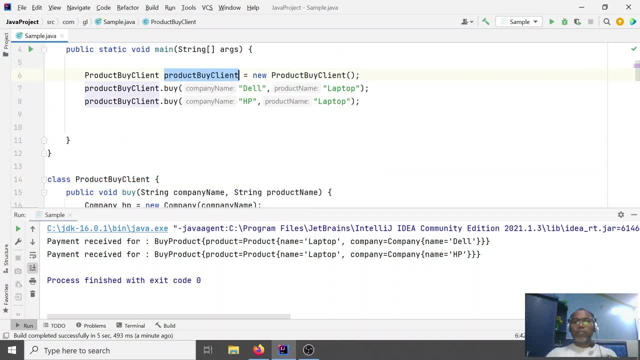 This client is a facade object. This facade object just create object and invoke the one method. And in this method you are creating a lot of company object, product object, buying object, payment, receipt, each and every things. but that doesn't need for any client. 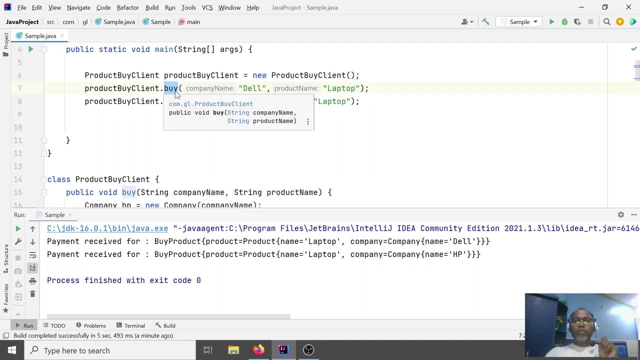 Whatever the input, your system need just only those input. you, your method, your client, your code take as input parameter So anyone can easily access your code and code is readable and easy to understand. Anyone can want to access your code. just create object and invoke one method. 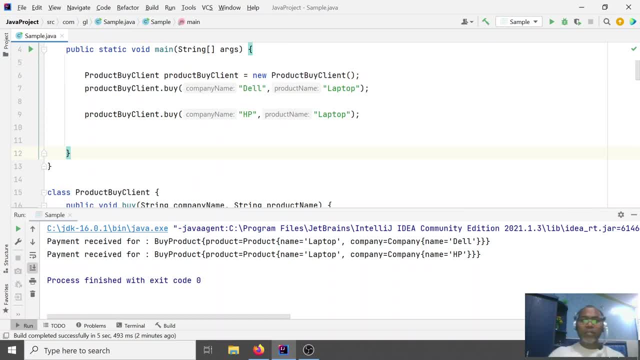 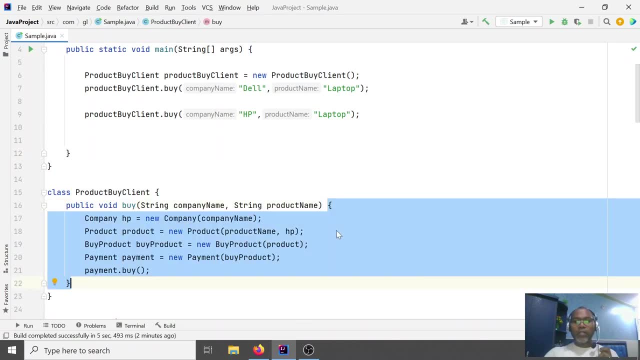 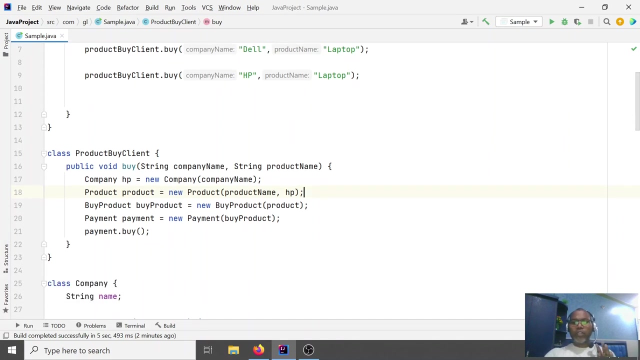 So this is the way facade is going to make your complex system Ok, Easy, are for use. So facade system is nothing not doing any kind of a business They don't want. you can change your business logic structure whatever you have. 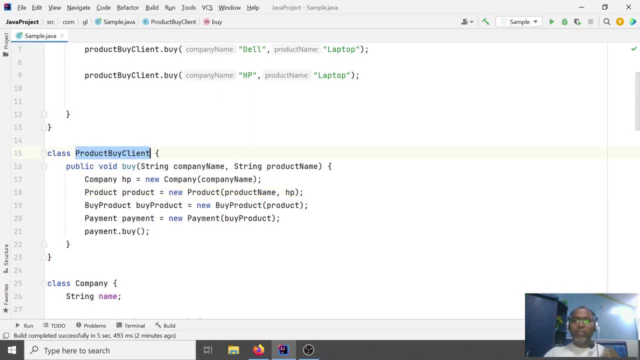 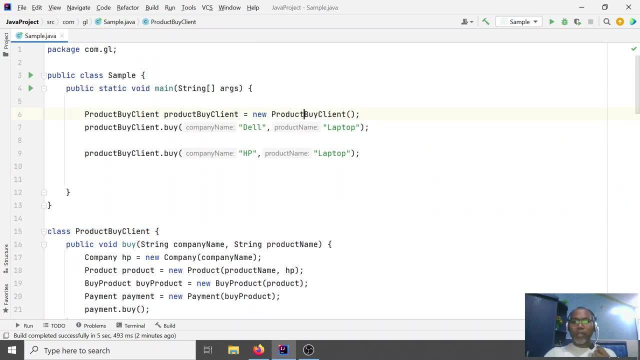 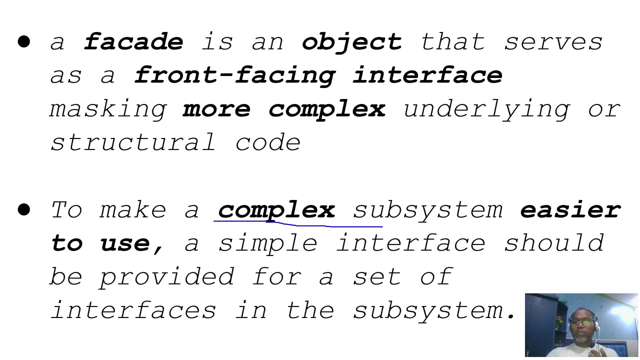 It's ok, Just add one more object. That is the client code. So anyone, any client, want to access your system, just use your client code. Client code: dot your function Done. That is the facade design pattern. So, facade design pattern: simply say whatever you have, your complex system or any system. 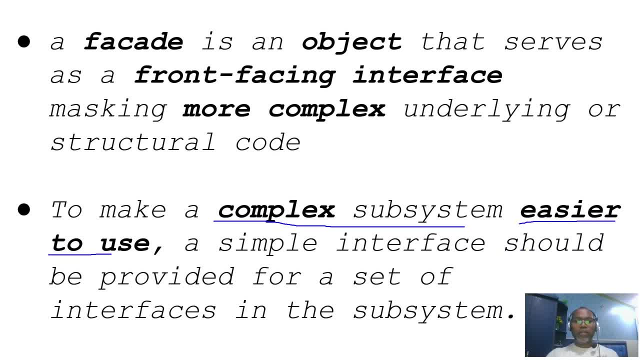 this make easier to use. Who use your system? client, customer, anyone? So this way, facade pattern. this is the facade pattern. Whatever your system, In which volume, Which order you want to, someone can use. You don't teach to each and everyone. 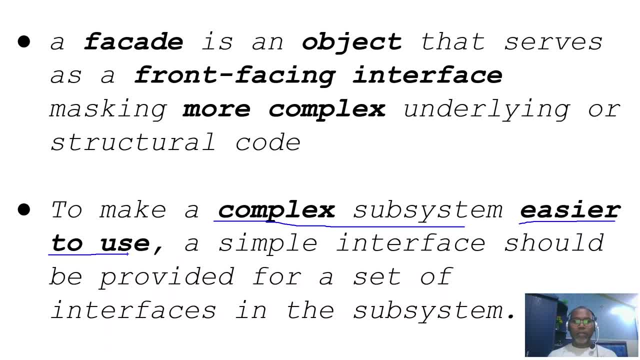 You can use my system: first this, create this object and that this object, and then this object. This logic you can just write in your facade object and expose facade object to the client And client can use simplified version of complex system. So this is the about your facade design pattern. 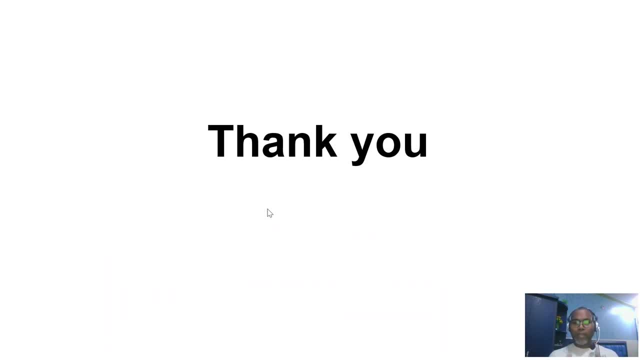 So now it's clear. Facade design pattern. just help your client can easier to access your system. As a software provider, this is our responsibility. Whatever our system we have designed, that is okay, working fine or the logic work correctly, But we have to also taken care who are going to use my software. 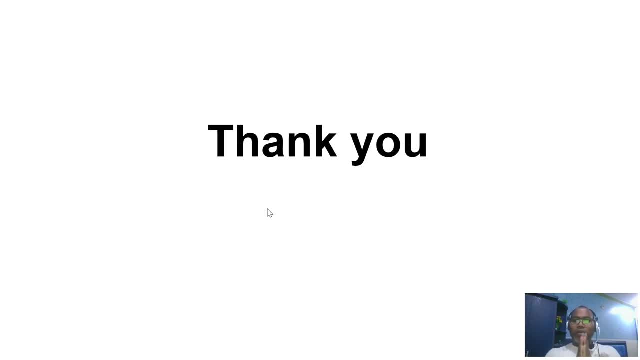 If someone going to use Those, you write one facade, one object. That is the simplified version Anyone can access. That is the facade Facade. just add one more layer for the client perspective. Now, first you design your system, Then you think how someone can use my system. 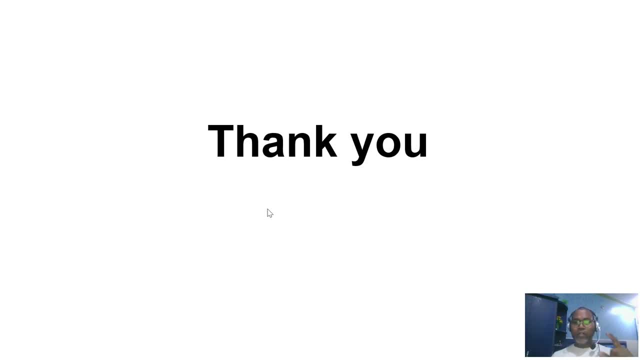 For those you write a client code. Client code is just simplified. Whatever the minimum input needed you take from client and rest of the structural things you do on your client code. So this is the simplified version. Client code is just simplified. Whatever the minimum input needed you take from client And rest of the structural things you do on your client code. 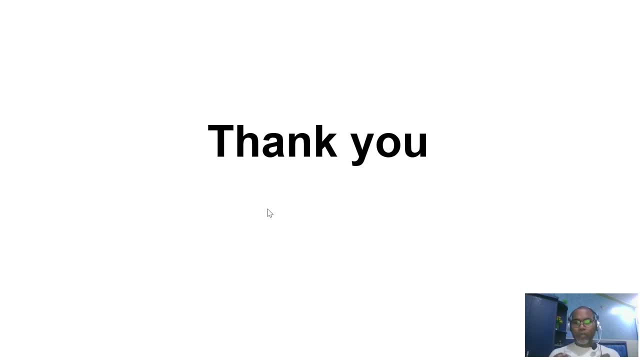 So this is the simplified version. Client code is just simplified, Whatever the minimum input needed you take from client and rest of the structural things you do on your client code. So hope it is easier. Facade design pattern, Facade object: make some complex system to more easier for you. 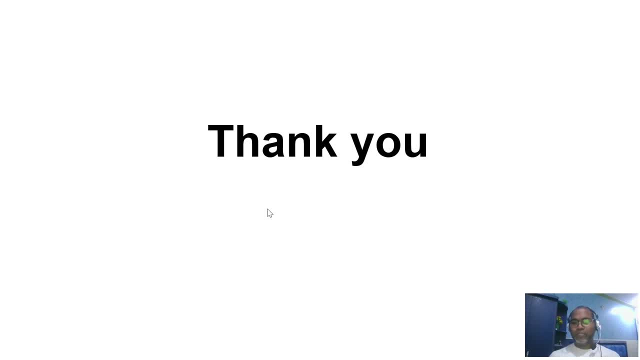 Facade object: make some complex system to more easier for you. So whenever you are writing any code, please be ensure you have to keep in mind for the customer. So whenever you are writing any code, please be ensure you have to keep in mind for the customer.